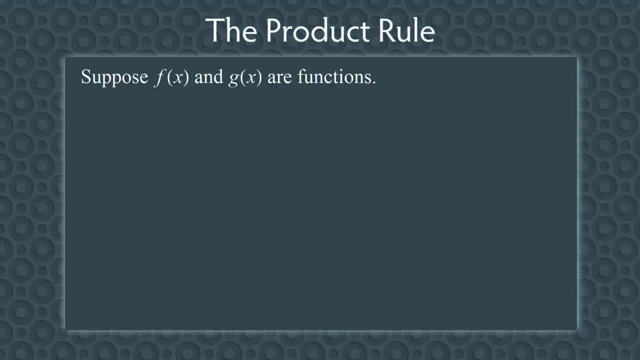 Suppose f of x and g of x are functions In arithmetic there are four operations: addition, subtraction, multiplication and division. For functions there are five fundamental operations: addition, subtraction, multiplication, division and composition For each operation. 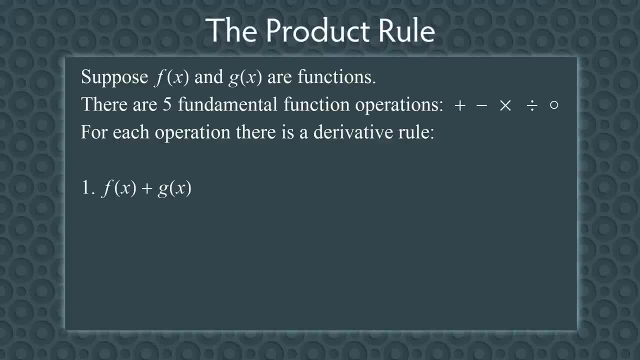 there is a derivative rule. If you add two functions together, you take their derivative using the sum rule. If you subtract two functions, you take the derivative using the difference rule. If you multiply two functions together, you take the derivative using the product. 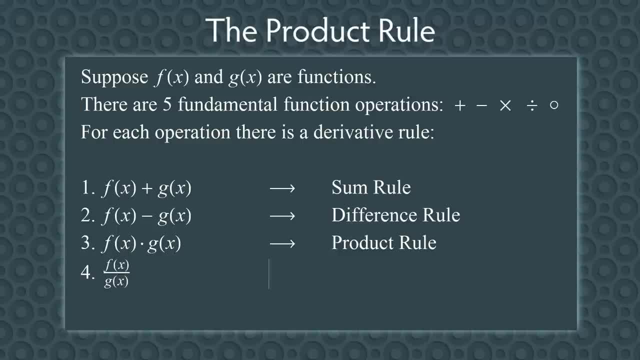 rule. If you divide one function by another, you take the derivative using the quotient rule, And for function composition you use the chain rule. Notice how the sum rule and difference rules are pretty straightforward. The derivative of a sum is the sum of the. 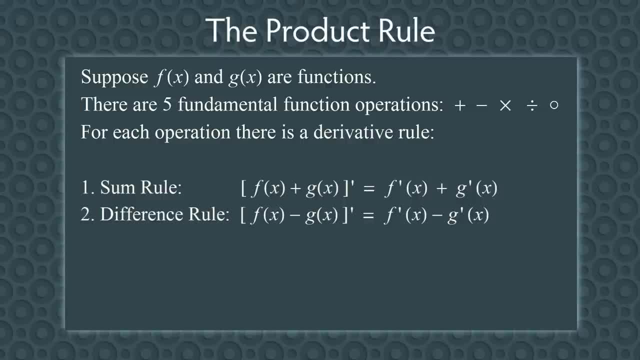 derivatives. The derivative of a difference is the difference of the derivatives. Sadly, this pattern doesn't hold for multiplication, division or composition. So today we're going to talk about the product rule. Let f of x and g of x be two functions. 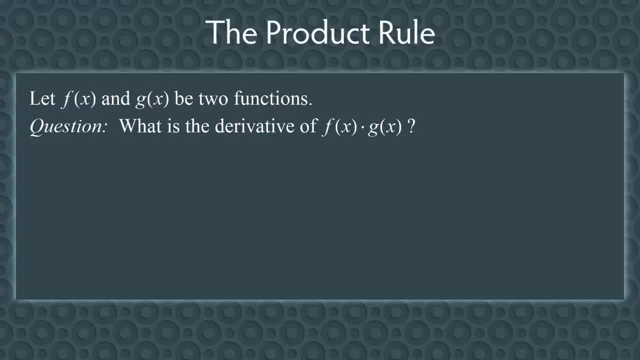 What's the derivative of f of x times g of x? This is given by the product rule. It says that the derivative of f of x times g of x is equal to the derivative of f times g plus f times the derivative of g. When working with functions, it's common to leave out the 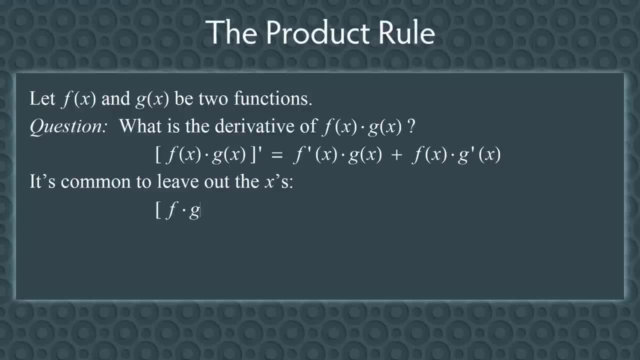 x's. If you do this, you get the derivative of f times g. So f of x times g equals f prime times g plus f times g prime. Don't forget that the derivative of f can also be pronounced as f prime. There are other ways to write the derivative f. 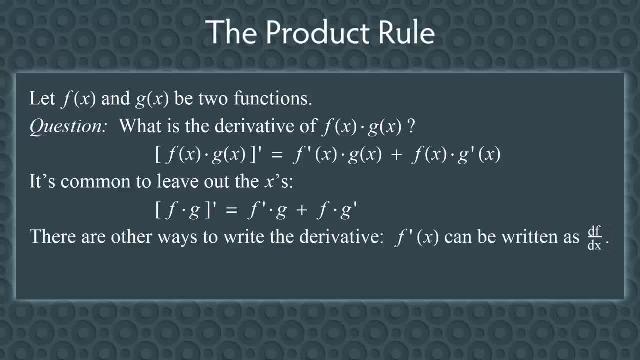 prime of x can also be written as df over dx. Using this notation, you get the derivative of f times g equals df, dx times g plus f times dg- dx. Notice the d over dx at the beginning. We call this an operator, and this operator means to take the derivative of everything. 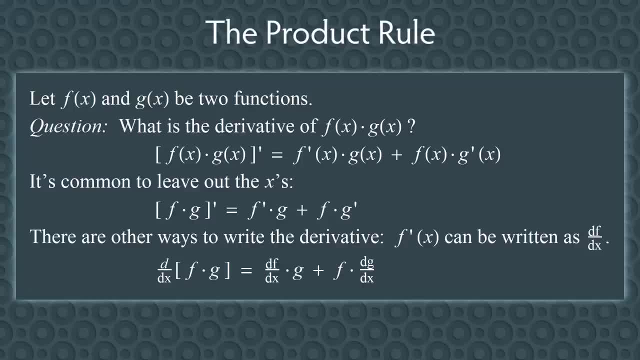 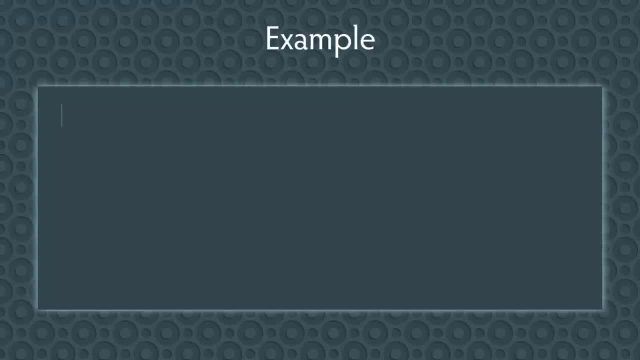 in the brackets. Here you have three different ways to write the product rule. They all say the same thing, only the notation is different. Let's see an example. Let's find the derivative of x squared minus 2 times 7x, cubed plus 5.. There are two ways to do this. One we can: 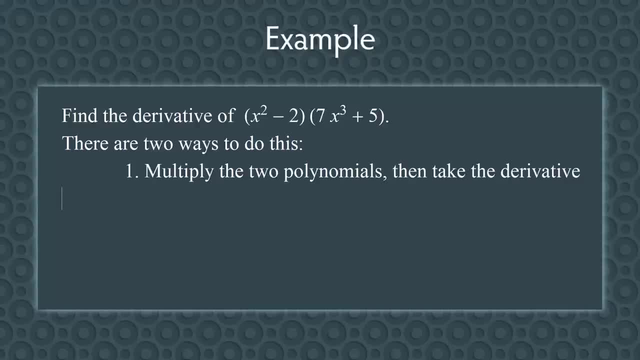 multiply the two polynomials, then take the derivative, Or two. we can use the product rule. We'll use both ways. First let's multiply the two polynomials and then take the derivative, so we'll know what the answer should be. Remember, when you multiply two polynomials together: 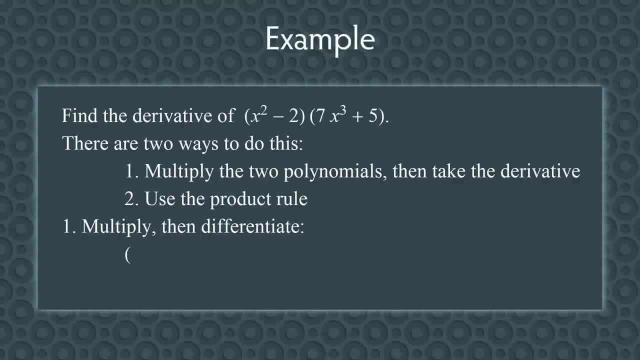 you multiply each term on the left by each term on the right, x squared minus 2 times 7x cubed plus 5 gives us: if we multiply x squared times 7x cubed, we get 7x to the fifth. 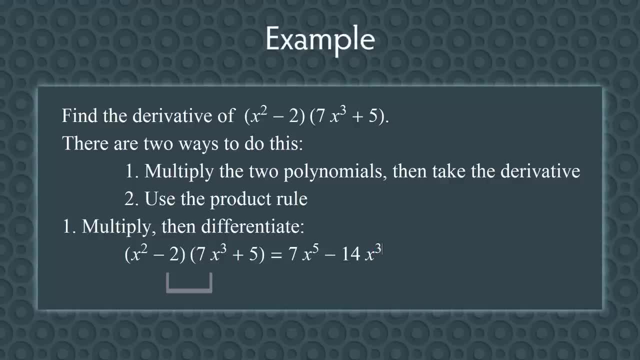 Negative 2 times 7x cubed is negative. 14x cubed x squared times 5 is 5x squared, and negative 2 times 5 is negative 10.. Let's now take the derivative of this polynomial. You do this term by term. The derivative of 7x to the. 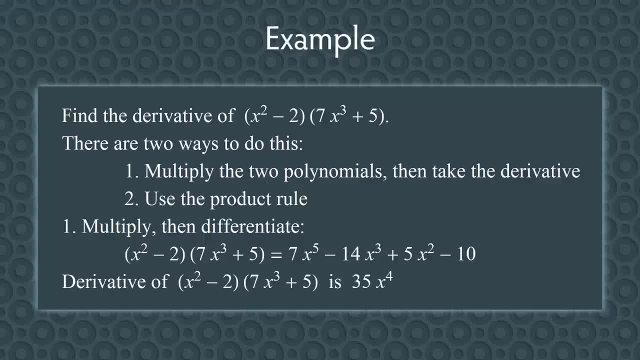 fifth is 35x to the fourth. The derivative of negative 14x cubed is negative 42x squared. The derivative of 5x squared is 10x and the derivative of negative 10 is 0.. Don't forget. 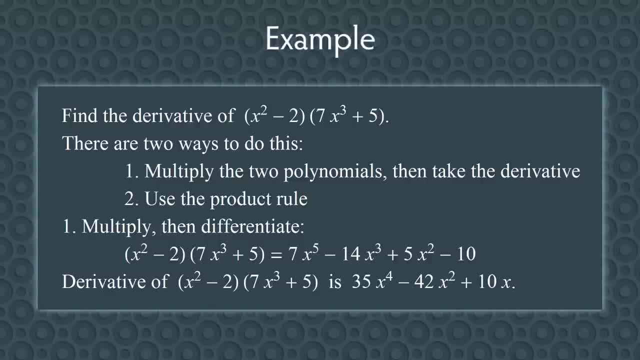 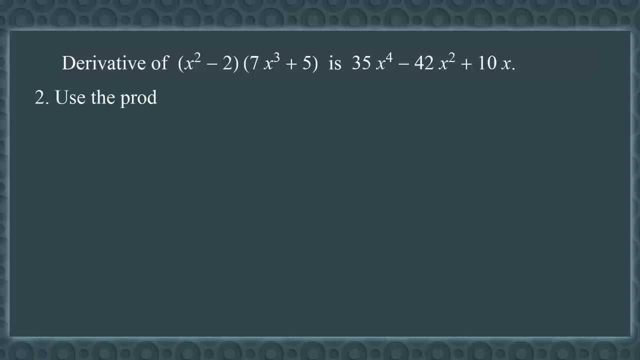 the derivative of any constant number is zero. So we get that the derivative of x, squared minus 2 times 7x, cubed plus 5, is 35x to the fourth, minus 42x squared plus 10x. Let's find the derivative again, but this time we'll use the product rule. 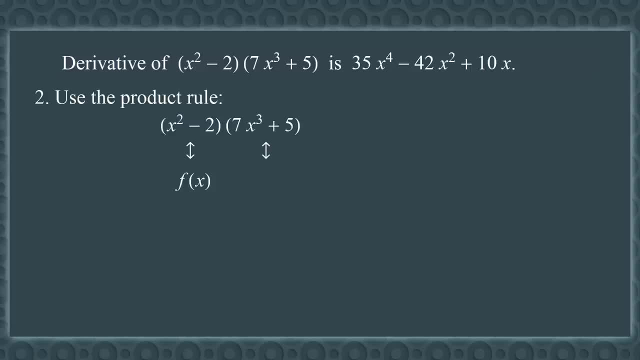 In this example, x squared minus 2 is f of x and 7x cubed plus 5 is g of x. Since f of x equals x squared minus 2, the derivative of – Write – into the derivative, you'll find x minus 2, y minus v minus…. 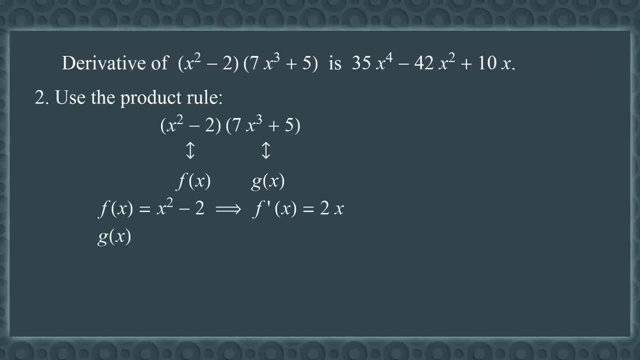 derivative of f equals 2x And g of x equals 7x cubed plus 5, so g prime equals 21x squared. We now have everything we need to use the product rule. Remember the product rule says that the derivative of f times g equals f prime times g, plus f times g prime. Now we 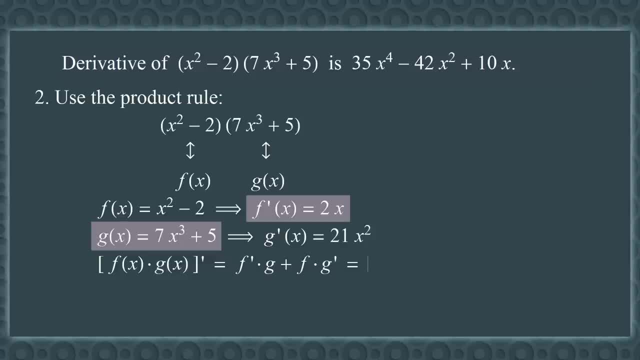 just plug in everything that we computed. so f prime times g is 2x times 7x cubed plus 5.. In the second term, f times g prime, if we plug everything in, we get x squared minus 2 times 21x squared. Now let's multiply these out and if we do that we get 14x to the. 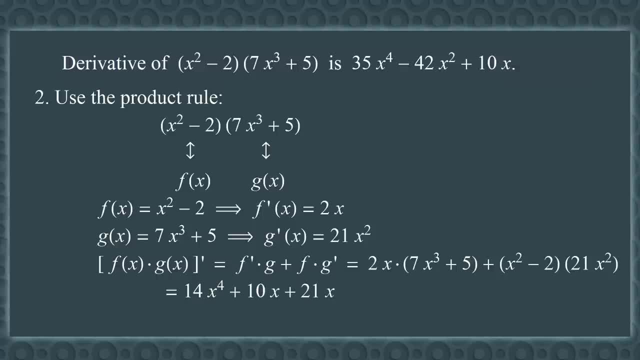 fourth plus 10x, plus 21x to the fourth minus 42x squared. If we combine like terms, we get 35x to the fourth minus 42x squared plus 10x. That's the right answer, Let's see. 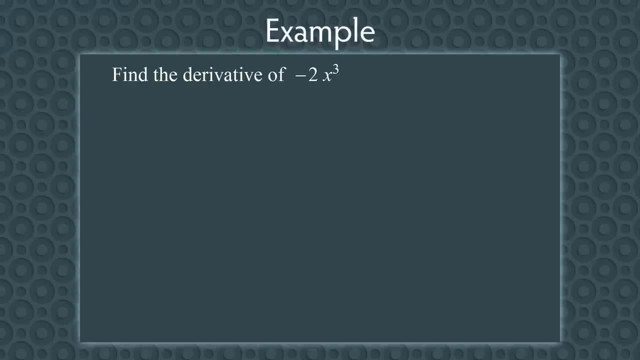 another example: Let's find the derivative of negative 2x cubed times sine x. First we have to decide what f of x and g of x will be. Let's group them. so negative 2x cubed is f and sine x. 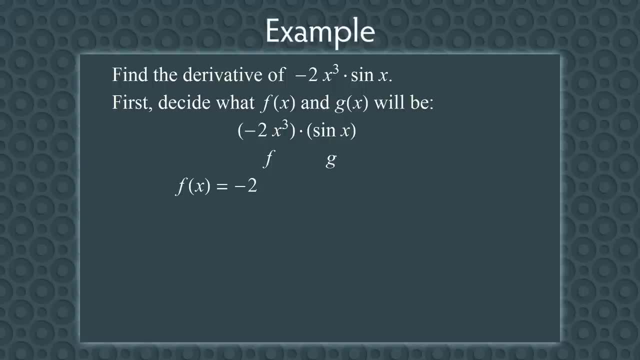 is g. Since f of x equals negative 2x cubed, the derivative of f is negative. 6x squared, g of x equals sine x. so g prime equals cosine of x. Let's now use the product rule. It says: 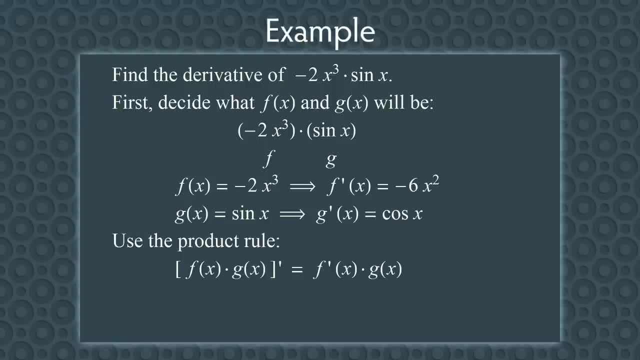 that the derivative of f is negative 6x squared and g of x equals sine x. so g prime equals 2x cubed. Finally, the derivative of f times g is equal to f prime times g, plus f times g prime. Now let's plug everything in For the first term: f prime times g, we get negative. 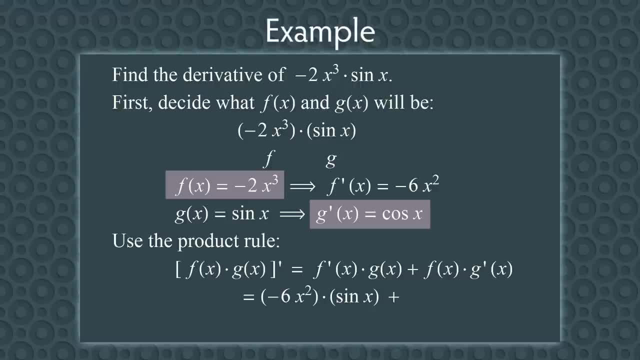 6x squared times sine x. and if we plug everything in to the second term, we get negative 2x cubed times cosine x. If we multiply everything now, get rid of the parentheses- you get negative 6x squared times sine x, minus 2x cubed times cosine x. There aren't any like terms, so we 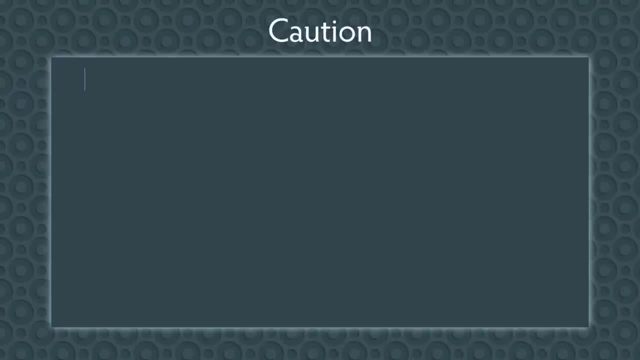 We can't simplify this any further Before we see a more complex example. I'd like to take a moment and talk about a common mistake people make with the product rule. People often make the mistake and say the derivative of f times g equals f prime times. 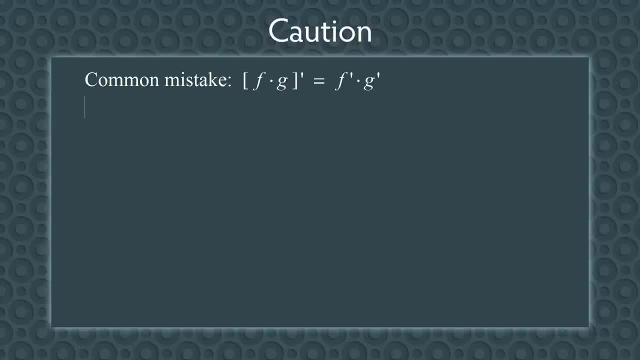 g prime. You can see where it's tempting to make this mistake. After all, the derivative of a sum is the sum of the derivatives, and the derivative of a difference is the difference of the derivatives. so you might think that the derivative of 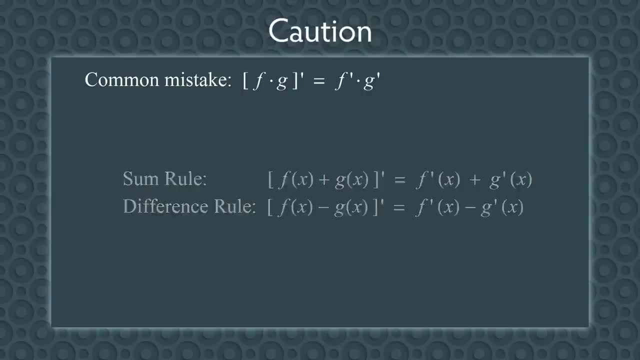 a product is the product of the derivatives, but this pattern doesn't hold. So how do you avoid making this mistake? Here's how: Write down what you think the formula is, then test it. And to test it, just pick two simple polynomials and try it out. 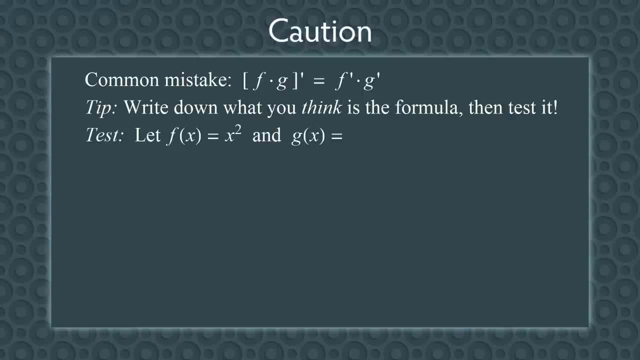 In this case, let f of x equals x squared and g of x equals x cubed. f of x times g of x is x squared times x cubed, which equals x to the fifth. So the derivative of f times g is just the derivative of x to the fifth, which equals. 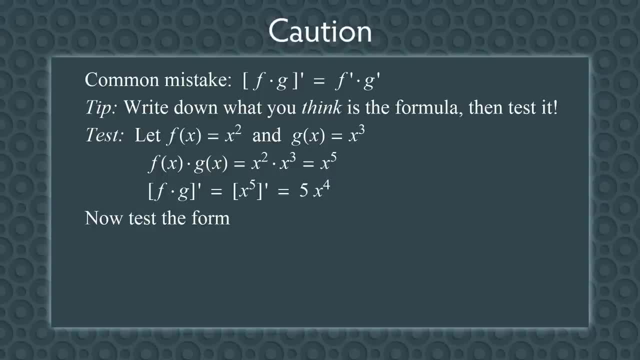 5x to the fourth. Now that we know the answer, let's test the formula. Suppose you think the derivative of f times g equals f prime times g prime. Let's plug everything in and see if this works. The derivative of x squared is 2x. 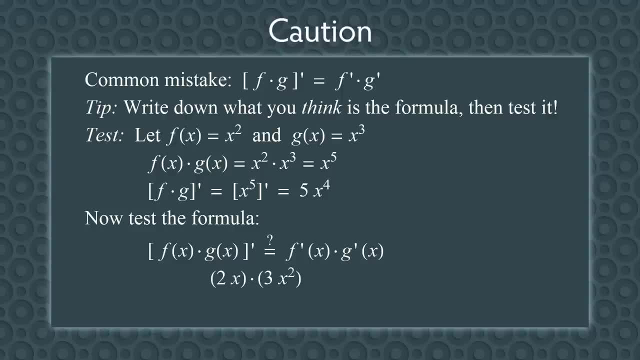 The derivative of g is 3x squared. If you multiply these together you get 6x cubed, But this is different than 5x to the fourth. So we know this formula is wrong. The derivative of f times g is not equal to f prime times g prime. 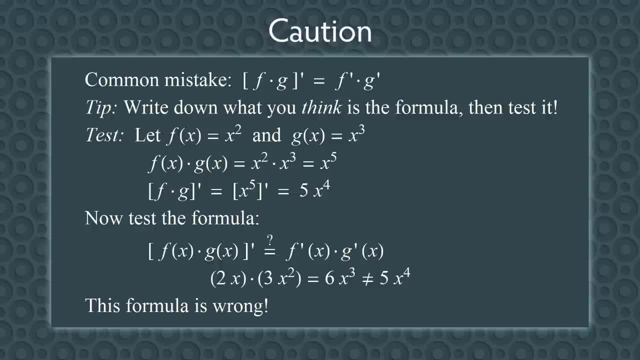 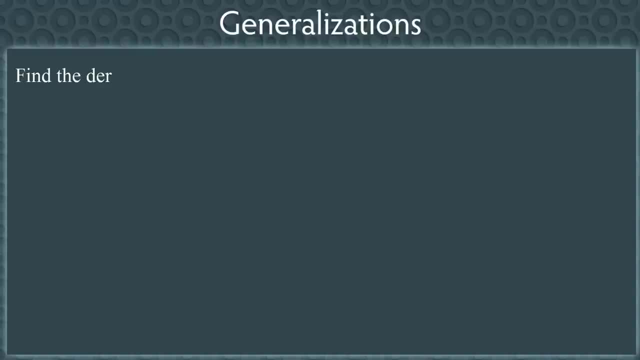 Whenever you're working from memory, it's a good idea to write down the product formula and quickly test it to make sure it's right. Let's now see a more complex example. Let's find the derivative of 17x times cosine, x times e to the x. 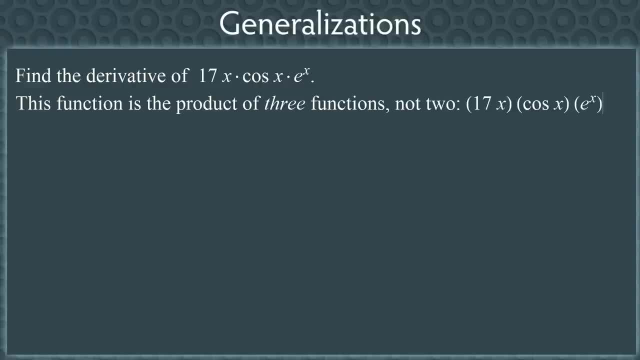 This is the product of three functions, not two, But the product rule only works for two functions. so what do you do? Here's the trick. We're going to use the product rule repeatedly. To see how to do this, let's find the derivative of f squared times g squared times g, prime. 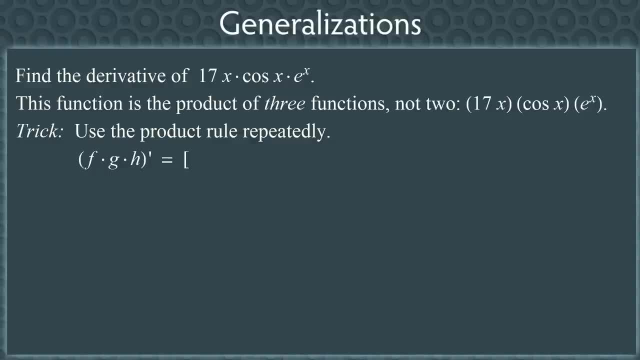 Let's find the derivative of f squared times g prime times g prime. It's f times g times h. What we're going to do is we're going to group f and g together and treat it like it's a single function. So the derivative of f? g times h is equal to the derivative of f? g times h plus f g. 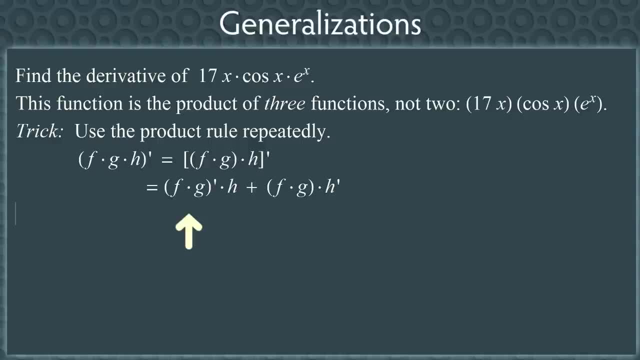 times the derivative of h. Next we're going to use the product rule again to find the derivative of f times g. The derivative of f times g is f prime g plus f g prime. If you multiply this out, you get f prime times g times h plus f times g prime times. 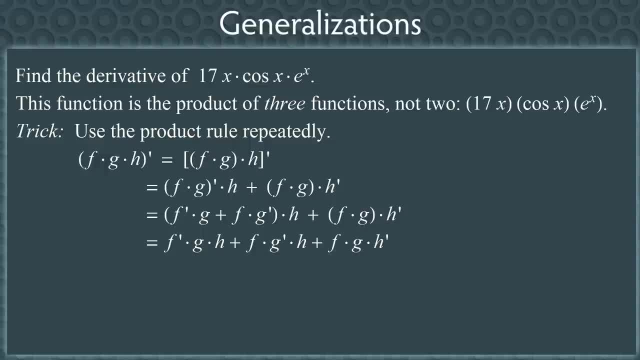 h plus f times g times h prime. This is the product rule for three functions. The derivative of f g h is equal to f prime g h plus f g prime. h plus f g h prime. Do you see the pattern On the right hand side? there are three terms. 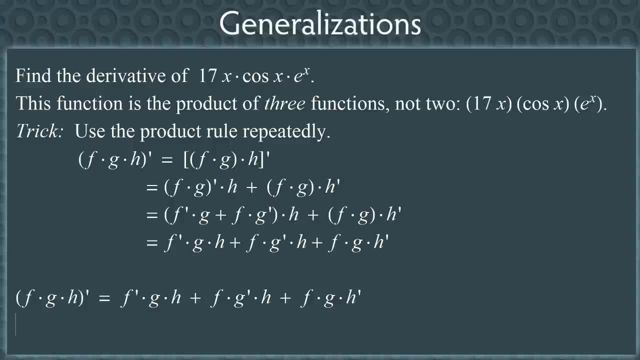 Each term has all three functions- f, g and h- and in each term you use the derivative of one of the functions. Since there are three functions, we need three terms so that the derivative of each function appears in one of the terms. 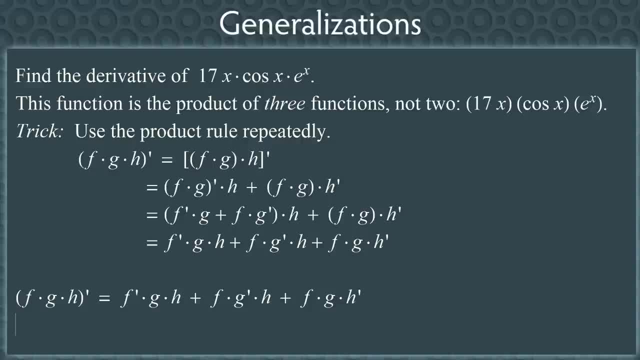 First f, then g, then h. This pattern also holds for four functions too. The derivative of a of x times b of x times c of x times d of x is equal to a prime, b, c d Plus a, b prime, c, d plus a, b c prime times d plus a, b, c, d prime. 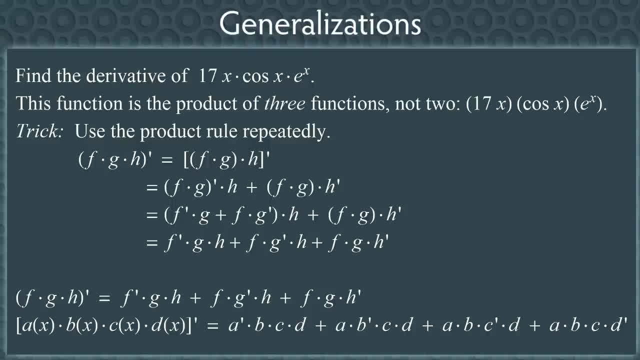 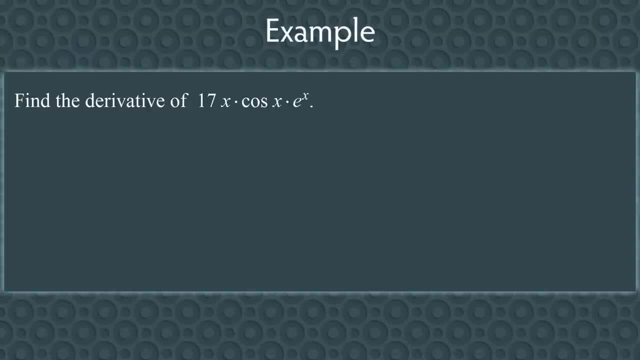 It's good practice to try and use the product rule three times to come up with this formula. Let's now solve the original problem. Find the derivative of 17x times cosine, x times e to the x. This is the product of three functions which we know how to differentiate. 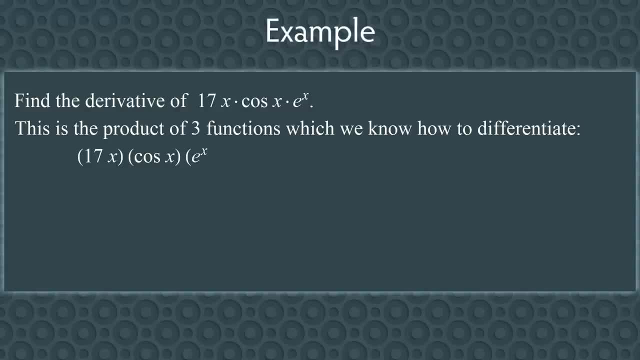 17x times cosine x times e to the x. So let f of x equals 17x g of x equals cosine x and h of x equals e to the x. Let's now use the product rule for three functions. The derivative of f times g times h equals f prime times g times h, plus f g prime h. 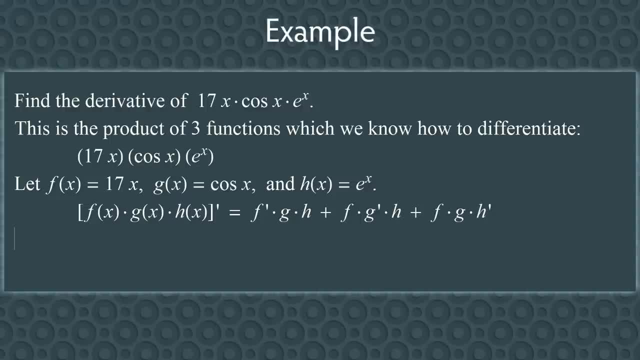 plus f, g, h, prime. Let's do this term by term. The derivative of 17x is 17.. So the first term is 17 times cosine x times 17.. Let's do this term by term. The derivative of 17x is 17 times cosine x times e to the x. 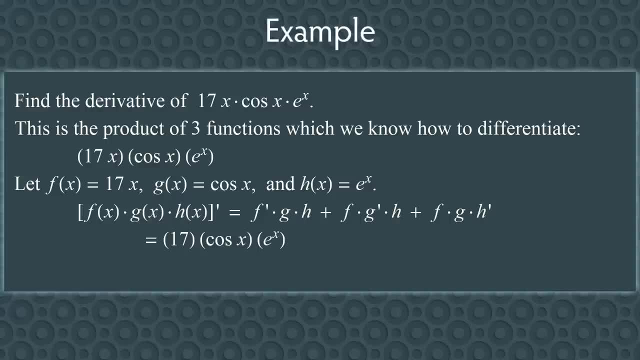 Next, we take the derivative of g of x, which is cosine of x. The derivative of cosine of x is negative sine x, So the second term is 17x times negative sine x, times e to the x. And finally, let's take the derivative of h of x: equals e to the x.